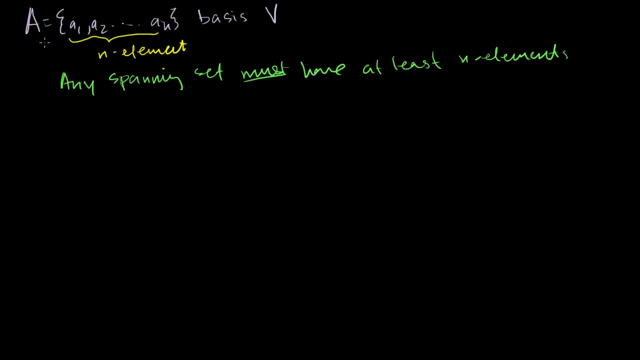 vectors in this set. So let's see if we could. if we have. I'm saying that every set that spans v must have at least n elements. if this sum basis set has n elements for v, Let's see if we can kind of run with a set that has less. 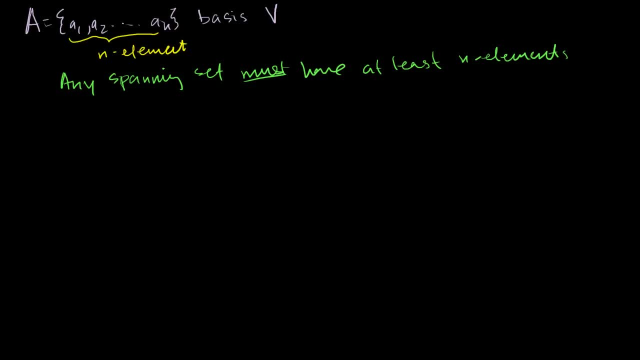 than n elements and see if we reach any contradictions. So let's say that I have some set b here and it's equal to the vectors b1, b2, all the way to bm, And m is less than n. so I have some set of vectors here. 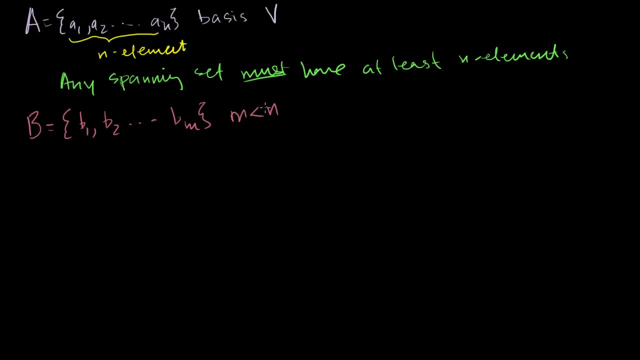 that have fewer elements than my set a, And let's say that b spans, that you come to me one day and you say, Look, I found you this set of vectors right here, and not only does it have fewer elements than a, but it spans. 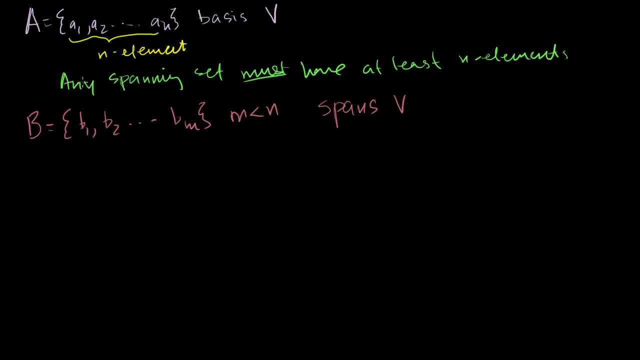 v, and I look at you very suspiciously because I always thought that this green statement was true. So we start a little bit of a thought experiment and I say: OK, you claim that your set spans v, so let's do something. 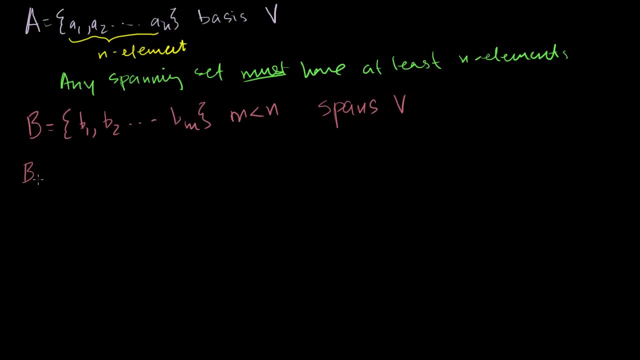 Let me define a new set. Let me call this new set b1 prime, and you'll see why I'm doing this kind of strange notation. It's essentially going to be is the set b plus my vector a1. So it's a1, and then I have all of my elements of b. 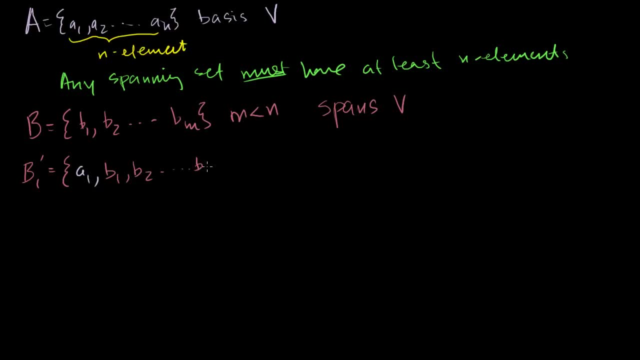 So b1,, b2, all the way to bm. Now I think you and I could both agree that this set is linearly dependent. How do I know that? Linear dependence means that at least one of the elements of the set can be represented as a linear. 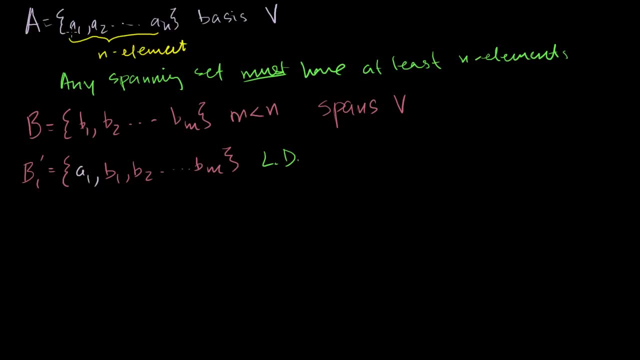 combination of the others. Well, we know that. a1. It's one of the basis vectors for v, for this definition of a basis. But all of the basis vectors are members of v right, You can obviously represent if this set is a basis for v. 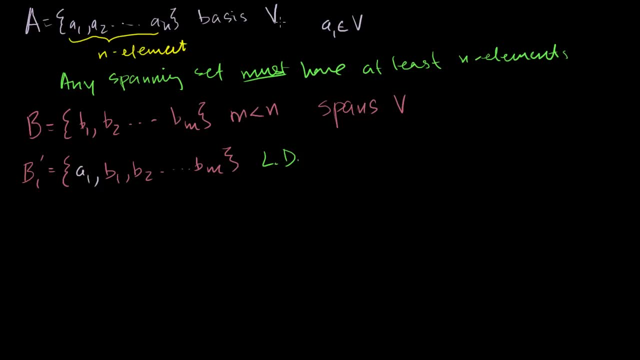 then this means that this set spans v, or that every member of v can be represented as a linear combination of these guys. Or another way is every linear combination of these guys is in v And one of the linear combinations of these guys is: 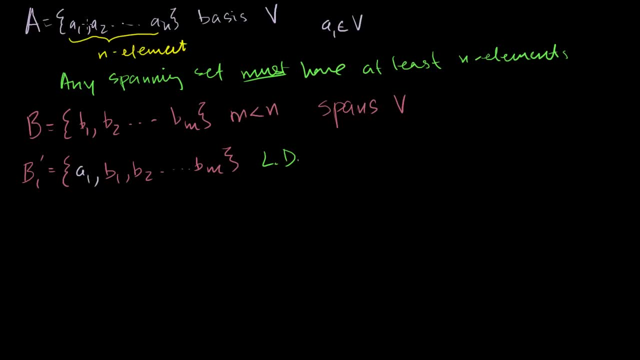 you just set the coefficient on a1 to b0.. The coefficient on a1 to b1, and the coefficients on everyone else to b0. So obviously a1 is also in the set. So if a1 is in v and all of these guys span v by, 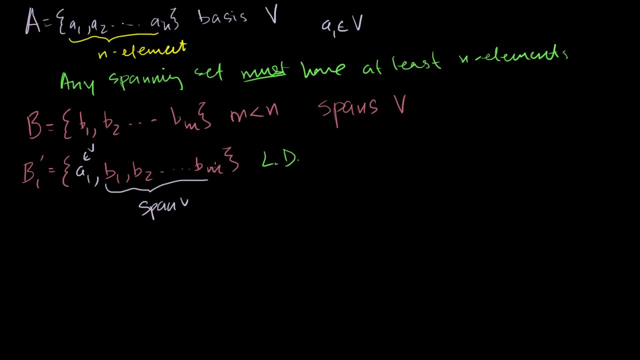 definition. if these guys span v, some linear combination of these guys can be used to construct any member of v. So you can take some linear combination of these guys to construct a1. So you could say a1 is equal to maybe d1, where the d's are the constants. 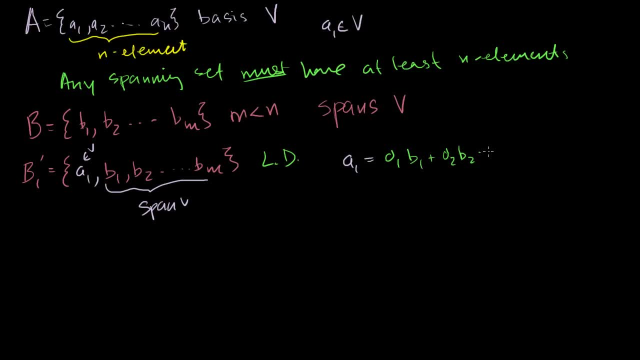 d1, b1, plus d2, b2, all the way to dm, bm, And at least one of these have to be non-zero. We know that a is a non-zero vector. If it was a zero vector, this couldn't be a basis, because 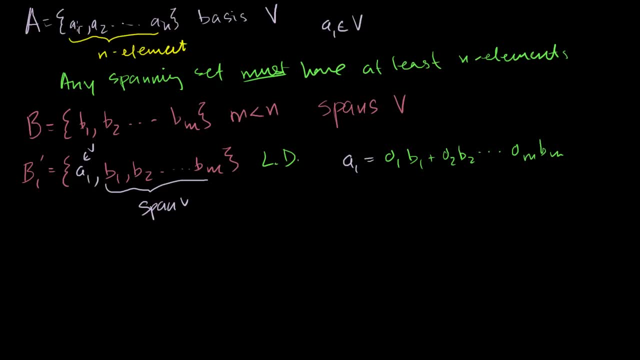 it wouldn't be linearly independent, Because you can always represent a zero vector as really just a zero times any other vector. So this won't be a zero vector. So at least one of these are non-zero. So let's just say: 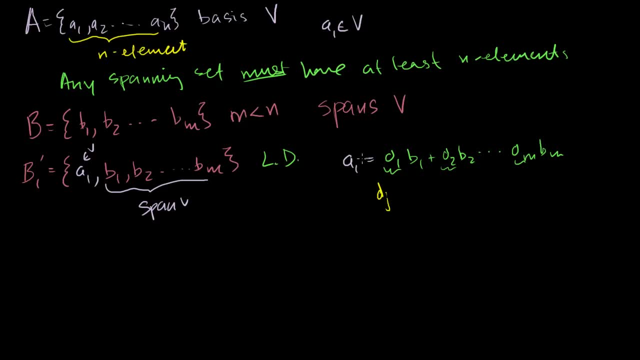 For the sake of argument, that dj. so the coefficient on bj is non-zero, So dj does not equal 0. So what we could actually do is we could solve for that term. So over here someplace you have the term dj, bj and it's plus. 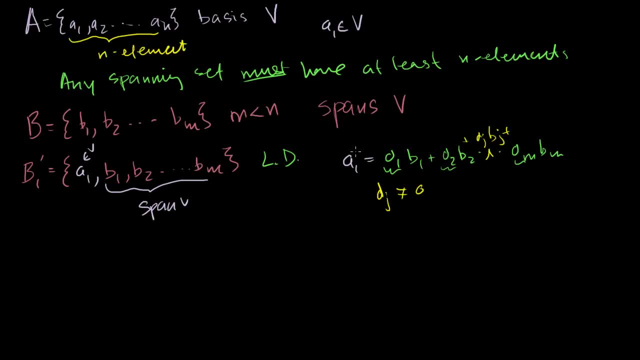 a bunch of other stuff We can solve for this term. if we subtract it from both sides of the equation and then divide both sides by minus dj and put this minus a1 on the other side, What do we get? I know that was a lot of operations, but that's just. 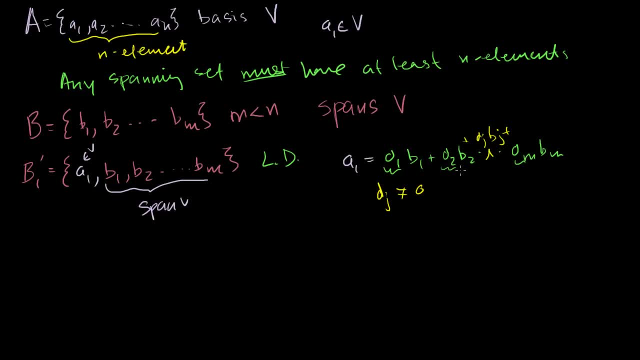 straight-up algebra, I think you can say that we could rewrite this right here. We can solve for bj, We could solve for our bj term and say that is equal to 1.. Sorry, that should be equal to minus 1 over its coefficient. 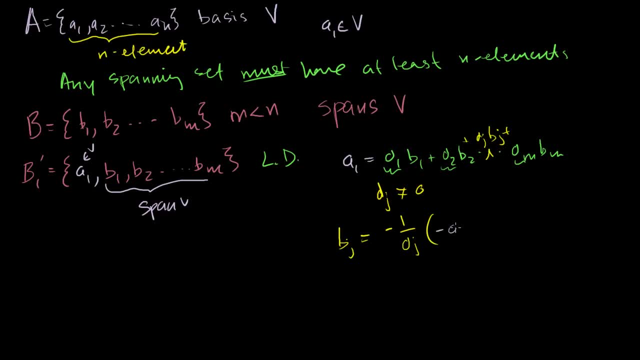 times, and if we subtract the a1 from both sides minus a1, and then plus all of these guys, plus d1, b1,, plus all the way, You're going to have a little bit of a gap here. I'll just draw it like that, this very unconventional 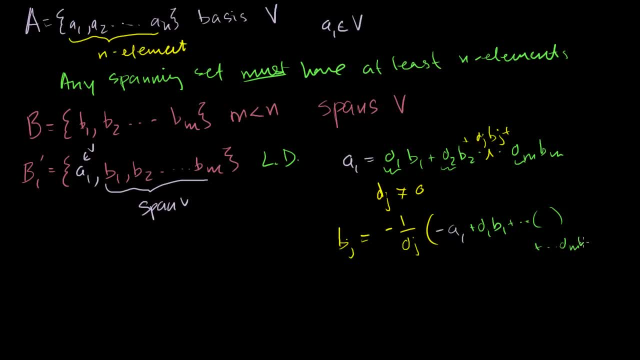 notation where this guy sat all the way to dm, bm. And I'm doing all of this just to show you that by definition, you can write a1 as a linear combination of these other guys. but you can just rearrange things. You can rearrange it so that you can write one of the other. 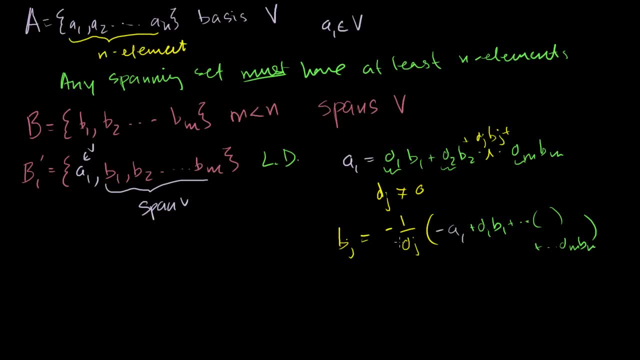 guys as a linear combination of the rest of the other guys and a1. And you say: you know what? This guy is now redundant. I don't need. I don't need this guy any longer to continue to span v. Clearly, this set still spanned v. 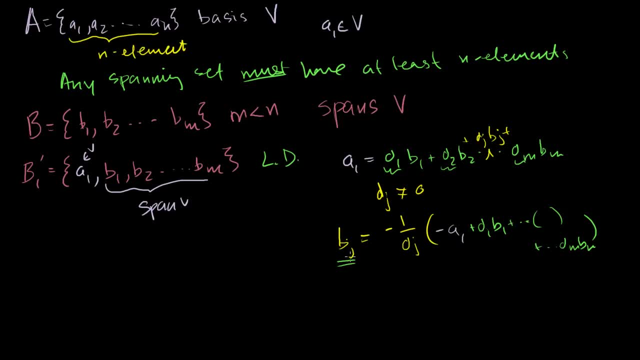 I mean, I added an extra vector here, But I can remove this guy right here. I can remove him from my set b1 prime and still span v. And how do I know that? Because I can achieve him by removing him, I don't lose anything. 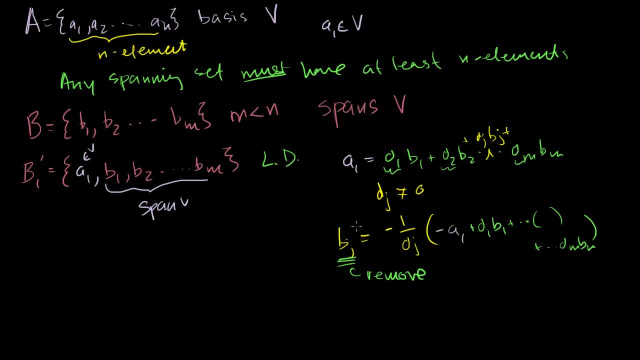 Because if I needed this vector to create some other vector, I can construct him with a linear combination of the rest of the b's plus my a1. So let's get rid of him and let's call that set b1.. And actually, just for the sake of notation, let me just change. 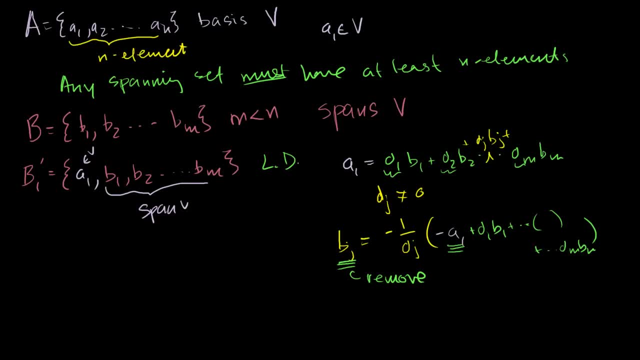 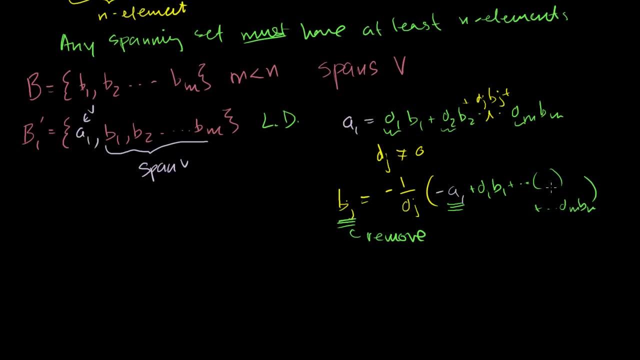 his name. This is a little unconventional. You won't see it done like this in any textbook, but I think it's a little bit easier instead of having to keep talking about these guys that are embedded someplace in the middle of the stream. 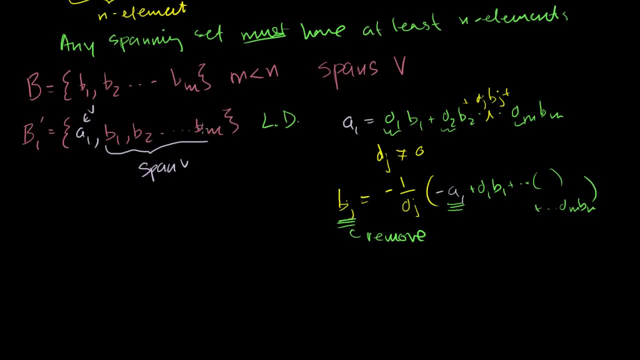 I mean these names b1,, b2, bm. they're arbitrary names, So let me just rename, Let me swap the labels. Let me just say that bj is b1.. b1 is equal to b1, and that b1 is equal to bj. 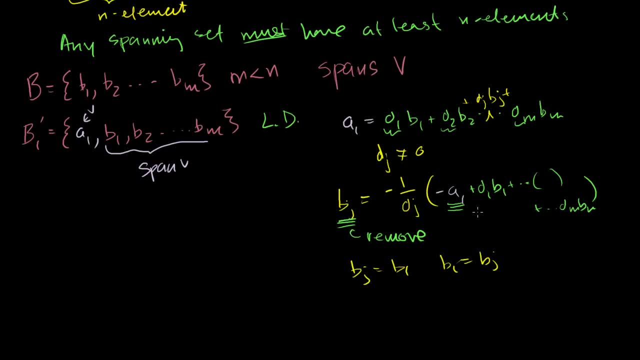 I'm just swapping their names, So I'm essentially just going to remove. I took that guy, I renamed him b1.. I renamed b1 bj so that I could swap them. So I'm essentially just going to remove b1 from the vector. 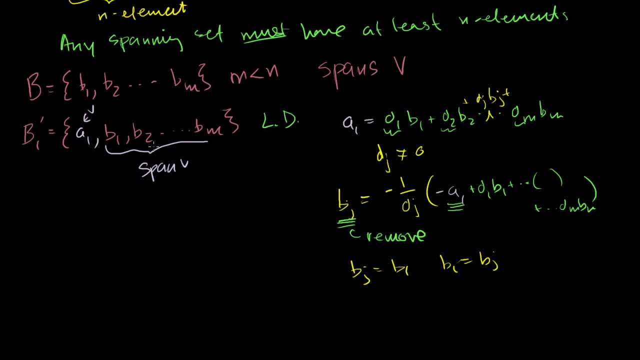 just to make my notation easier, You could just keep saying, oh, I'm going to remove this bj from the middle, but it becomes very confusing then. So let me call my new set after removing the bj that I've renamed as b1.. 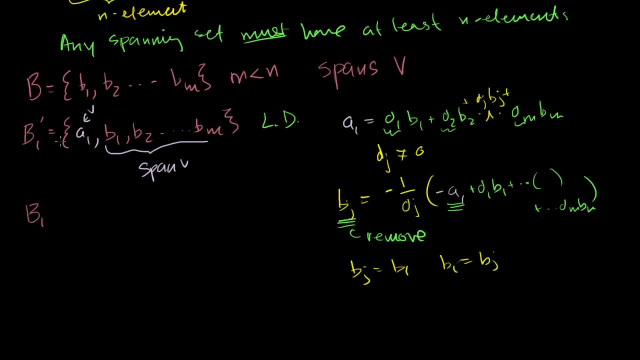 Let me just call that Straight up b1.. So my straight up set b1 is equal to a1.. And then, remember, I removed the bj and I renamed that as b1, and then I renamed b1 as bj. So now my set looks like this: 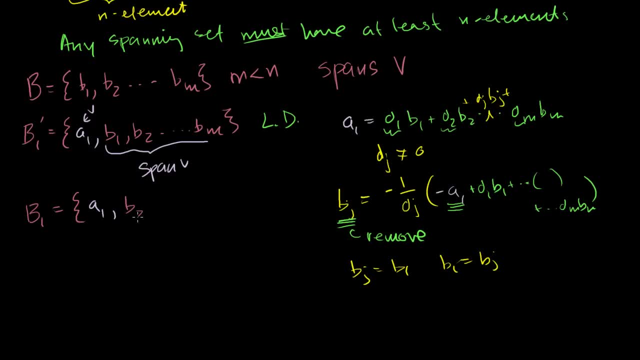 Let me go to the other color, b2.. And for all we know, bj might have been b1. We don't know, And there's probably multiple of these that are non-zero, So we could have picked any of those to be our bj. 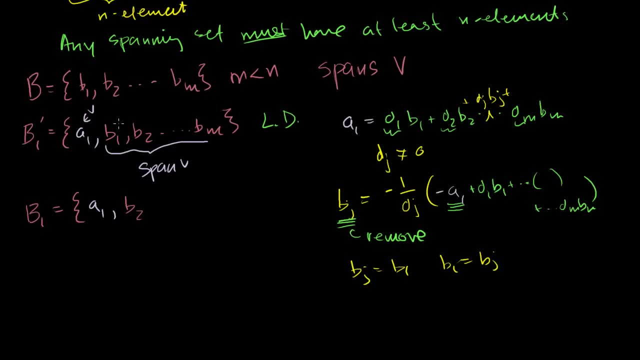 But anyway, We've got a set. We've got a set, So we took our bj, renamed it b1, and removed the b1. And so now our set looks like this: b3 all the way to bm. And this will still span. 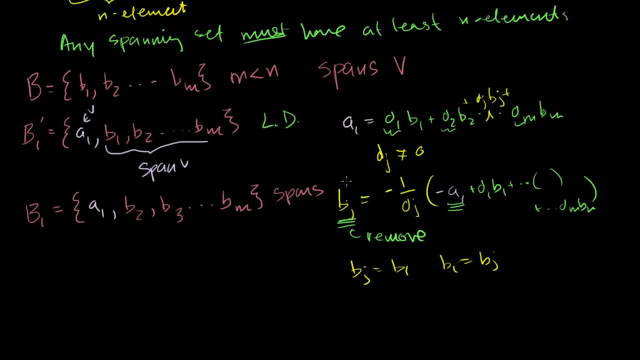 This set still spans v, And we know that because the guy we removed can be constructed with any linear combination of these guys. So we haven't lost our ability to construct all of the vectors in v. Now let me create another vector. Let me create the vector b. 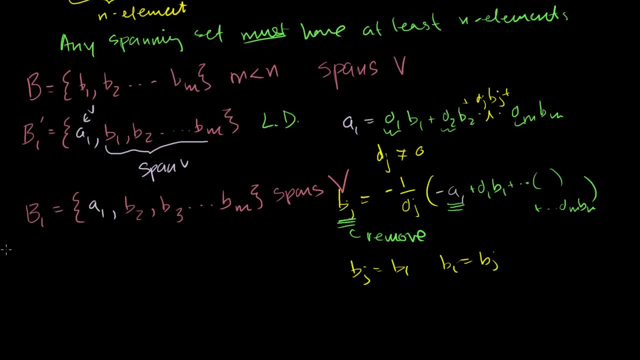 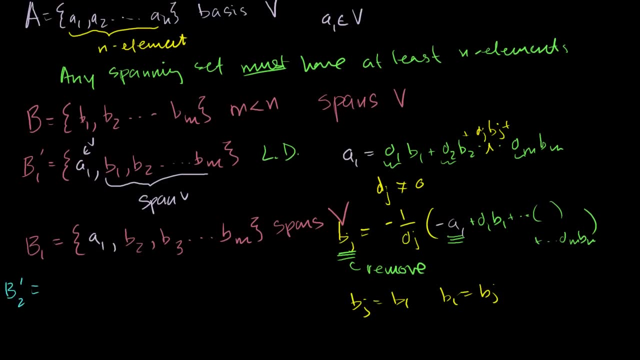 Let me do it in a new color. Let's say, I have the vector b2 prime And what I'm going to do here is now I'm going to take another element from our spanning, from our basis of v. I'll take the second element. 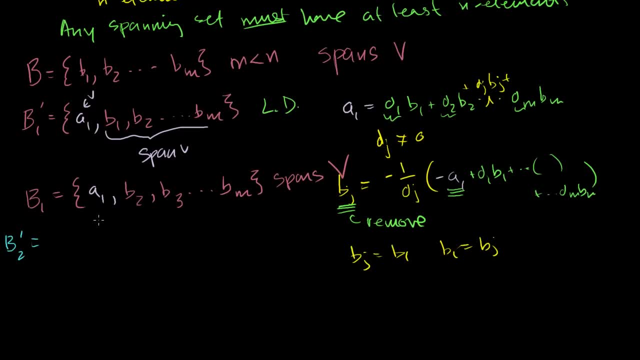 I'll take a2.. I'll take a2 and throw it on this guy. So now we have the set. Let me write it this way: b2, prime is equal to. I'm just going to add a2 to this guy. 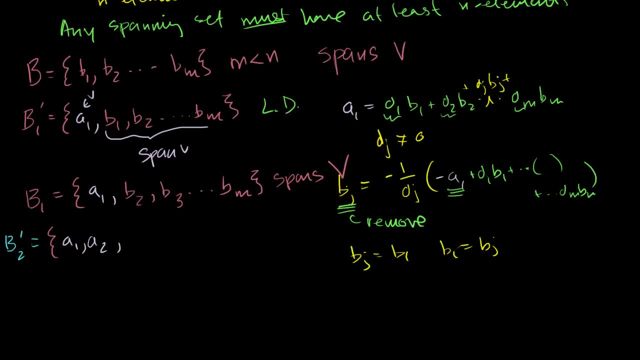 So you have a1., a2. And then you have all the rest of these guys: b2,, b3,, all the way to bm, And of course this still spans v. I just added something here, But this is definitely linearly dependent. 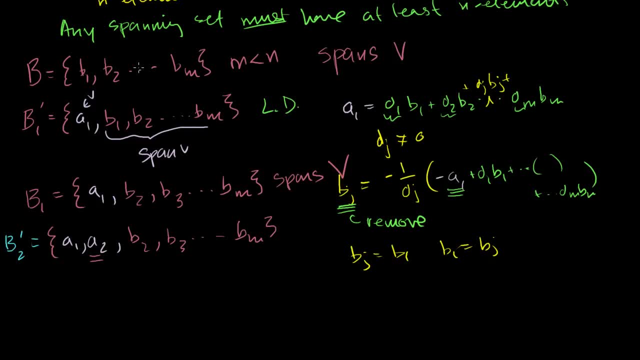 Remember I didn't say in the beginning whether this was linear dependent or not. It may or may not be, But when you add this other vector that's in v, you definitely know that you're linear dependent because these guys can construct that guy. 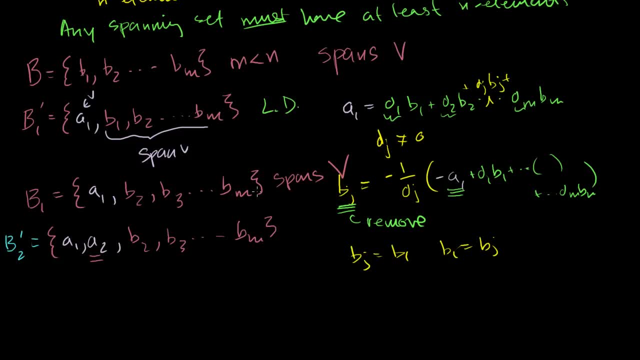 Similarly, we know that this vector b1, this spans v. So when we add this new element here, we know that it can be written as a linear combination of the other ones. So we know that this right here is linearly dependent. 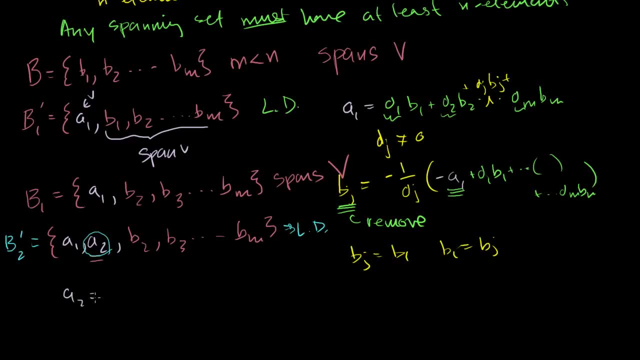 And we could say that a2 is equal to some constant times c1 times a1, plus- let me put some constants- so plus d2.. Actually, let me just write it this way, Since plus c2, b2,, plus c3, b3, all the way to cm. 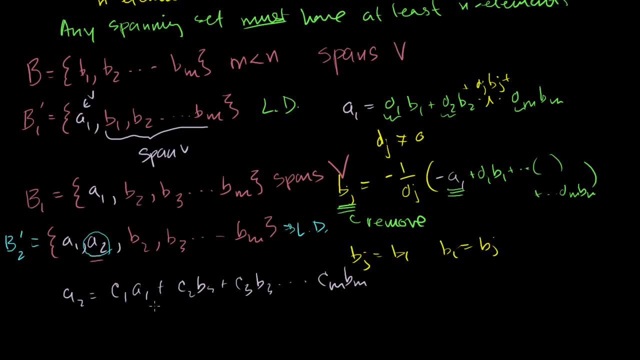 Now what I'm going to claim is that at least one of these coefficients is non-zero, So at least one of the ci's does not equal to 0. And I'll make the further claim that there's at least one that's outside of this one. 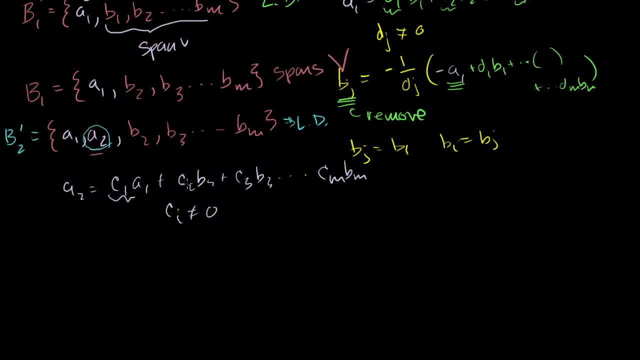 There's at least one that's outside of that one, That at least one of the coefficients on these b's, on these b terms, has to be non-zero. And the way you can kind of think about it is: what if all of these guys were 0?? 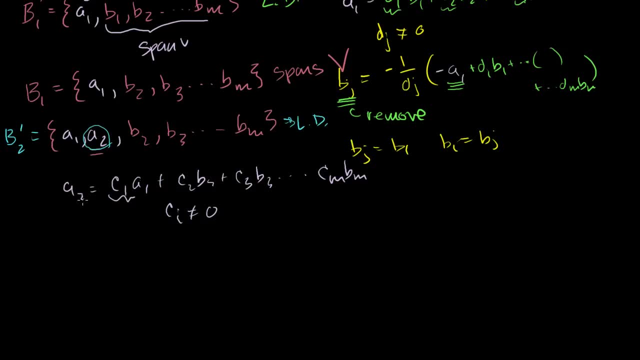 If all of these guys were 0, then that means that a2 is a linear combination of a1, right, All of these guys would cancel out and you'd have: a2 is equal to some non-zero constant times a1. But we know that's not the case, because these two guys 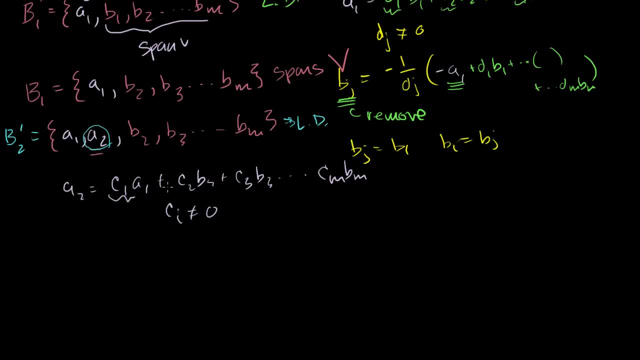 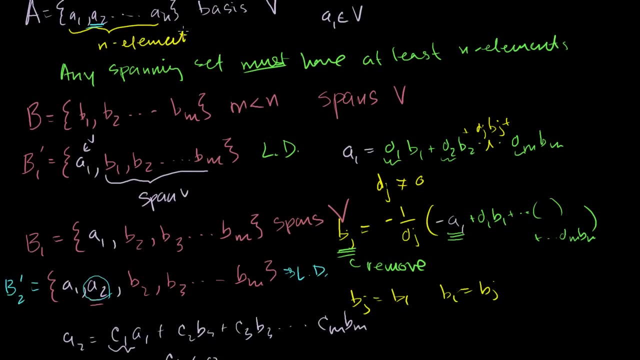 come from the same linearly independent set. They both come from that spanning basis. The fact that they are a basis, the word spanning basis- I shouldn't say it like that because it's redundant- A basis is a spanning set that is linearly independent. 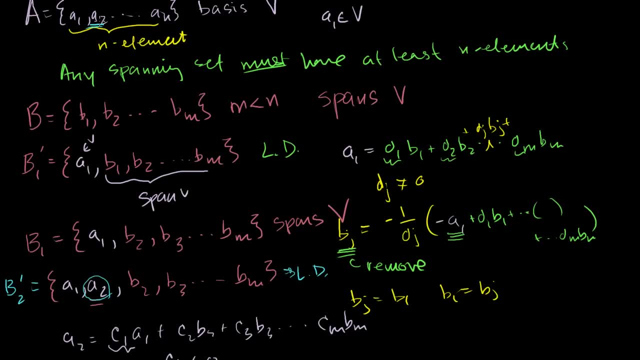 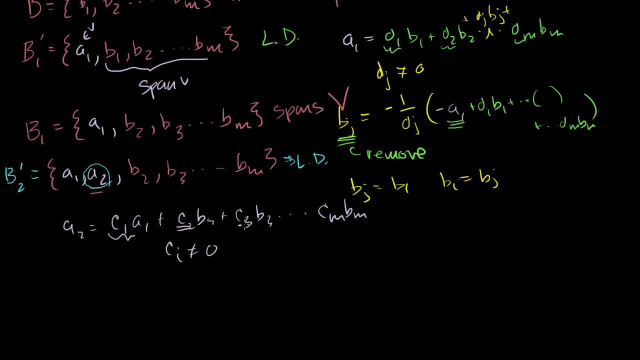 If they're linearly independent, then they're linearly independent. We know that a2 cannot be represented as some linear combination of the rest of these guys. So we know that one of the coefficients on the b terms has to be non-zero. 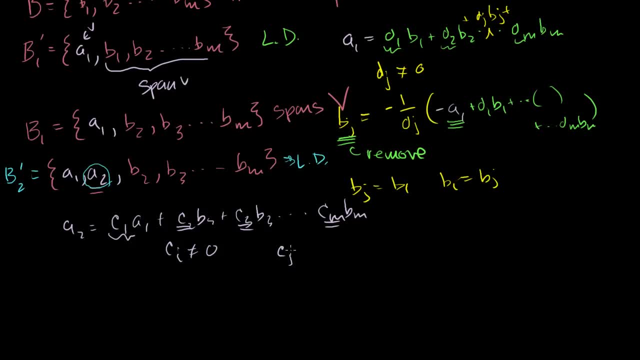 And once again, let's just say that it's the coefficient. someplace here you're going to have a cj bj. This is a different one than we had before, And we know that this guy- one of them, at least one of them- 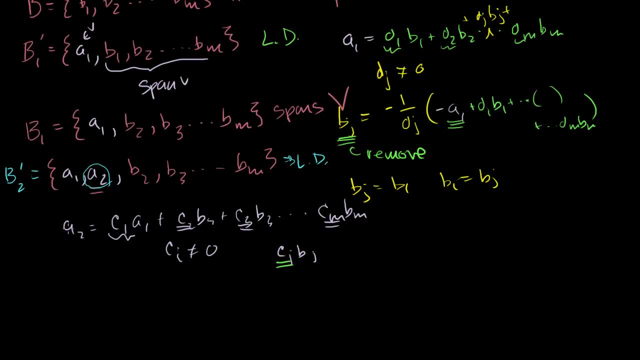 has to be non-zero, Because if all of these guys were non-zero, then you wouldn't be able to say that this vector and that vector are linearly independent, Because they would be scalar multiples of each other. So we're going to do the same exercise. 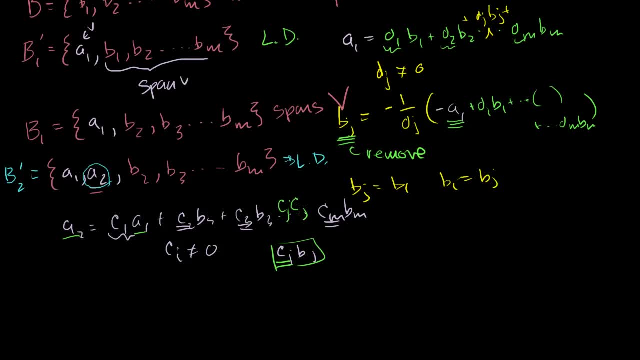 This guy right here. that's someplace. cj bj right here. Obviously, this coefficient is non-zero, So we can solve for our bj. Once again, we can say that bj is equal to minus 1 over cj times. now it's minus a2 plus c1, a1, all the way to cm. 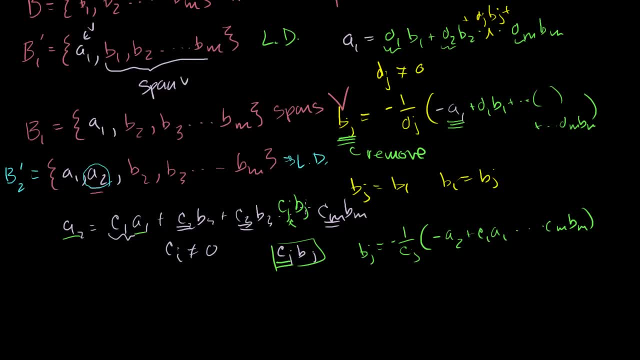 So we have some bj here that can be represented as a linear combination of the rest of the people, including our new a2.. And so, just like we did before, let's remove him, Let's take him out of the set, And before I take him out of the set, I'm going to rename. 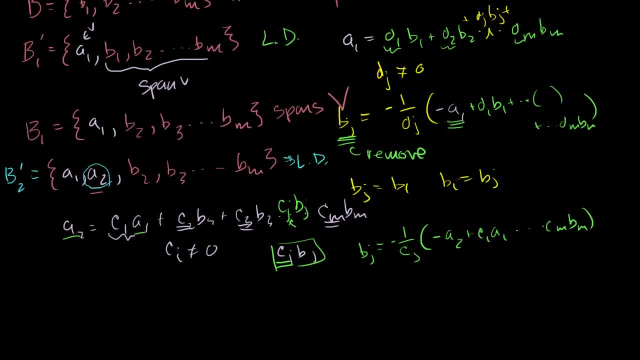 him. just solely for the purpose of notational simplicity, I'm just going to rename our bj b2.. And our b2 is equal to bj. So I'm just rearranging the names And I'm going to remove our b2.. 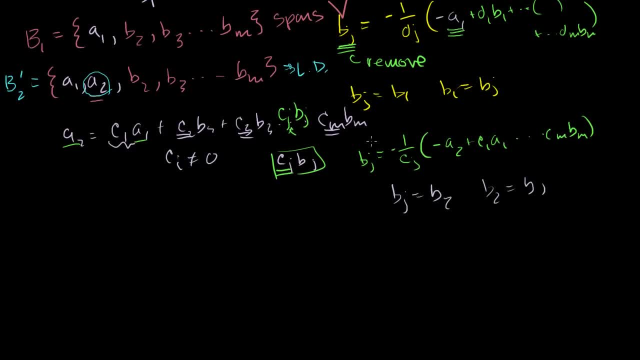 Or I'm going to remove what I now call our b2.. It was whatever was out here that could be represented as a linear combination of everything else, including our new a2. So let me call that set. When I remove one of those terms right here and now, I 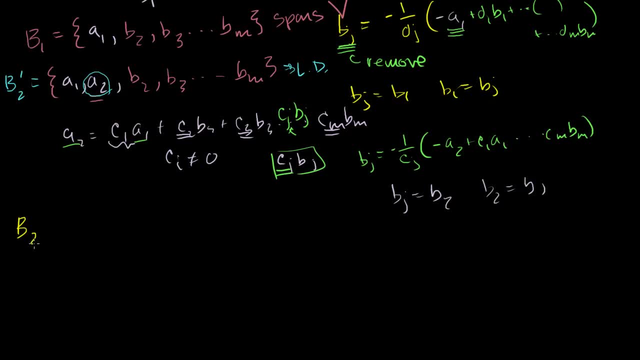 renamed it b2, I call this set b2. And now it's equal to a1, a2. And now I have the leftovers Of my b's, So I have b3,, b4, all the way to bm. 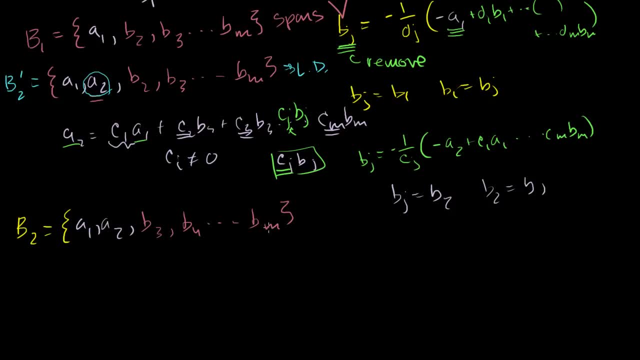 I notice I still have exactly m elements And this still spans. So this spans v. It spans v because the element that I took out of it can be represented as a linear combination of these guys. So if I ever want to construct anything that needed that I 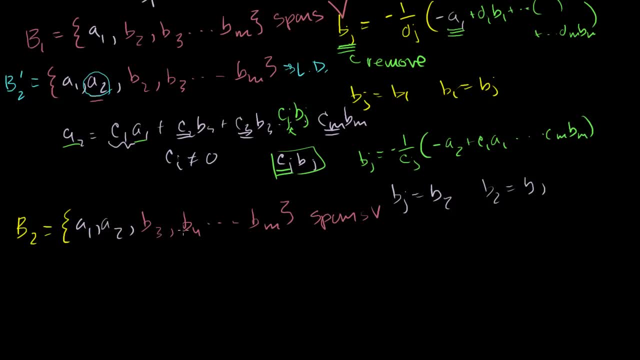 can construct that vector with some combination of these guys. So it wasn't necessary. So it still spans v. So this process I'm doing, I can just keep repeating it. I can add an a3.. I can define b3 prime. as I can just add a3 to this set, right. 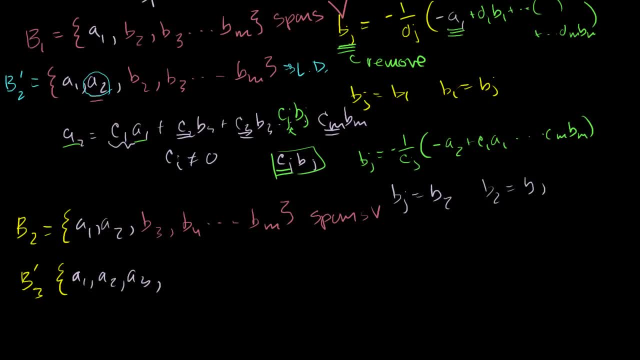 here a2, a3. And then I have my b3, b4, all the way to bm And I'll say, oh, this is linearly dependent because this guy spans v. So everything but this guy spans v. 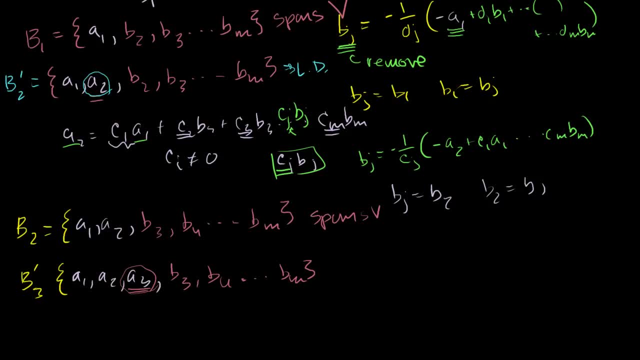 So obviously you can construct this guy with a linear combination of the rest of them. So you could say: a3 is equal to some a1 plus some a2, plus c3, b3, all the way to cm bm. And we know that at least one of the coefficients on the b 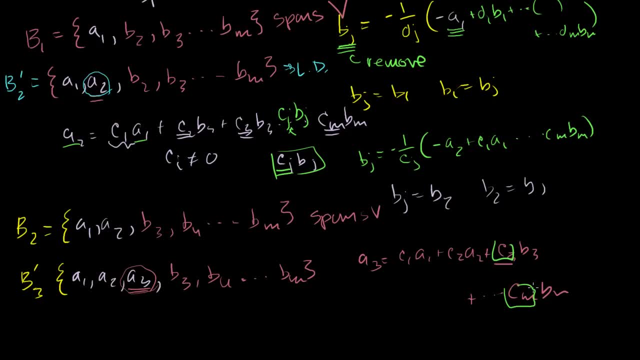 terms has to be non-zero, Because if all of those were 0, then you would be saying that a3 could be a linear combination of the a terms. And we know that a3 can't be represented as a linear combination of the a terms because all these a terms come. 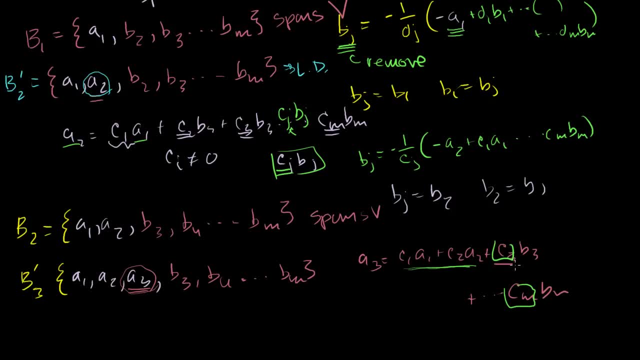 from a linearly independent set. So you do the same operation. You find you can solve. let's say that cj some term. right here the cj is non-zero, Then you can solve for that bj. And then I do that little renaming thing. I do where I. 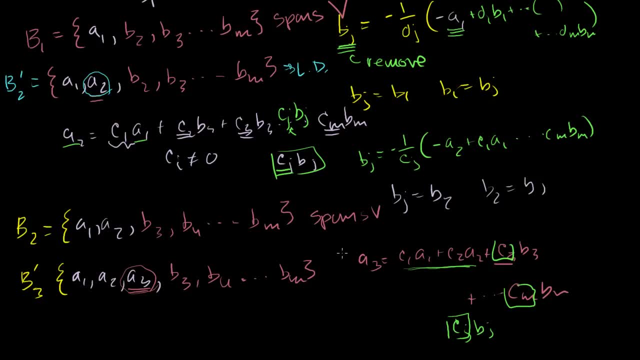 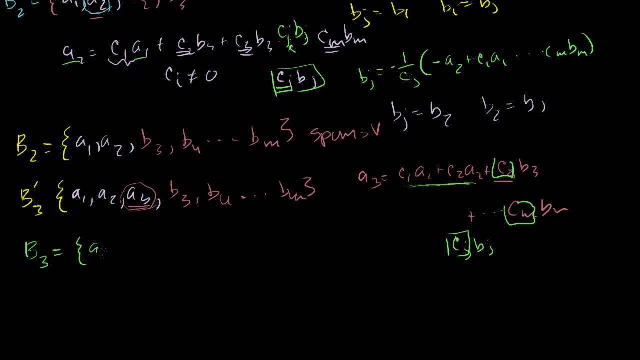 rename the bj b3 and rename b3- bj, and then I remove b3. And I get the set: b3 is equal to a1, a2, a3. And then I have b4 all the way to bm, And this still spans v. 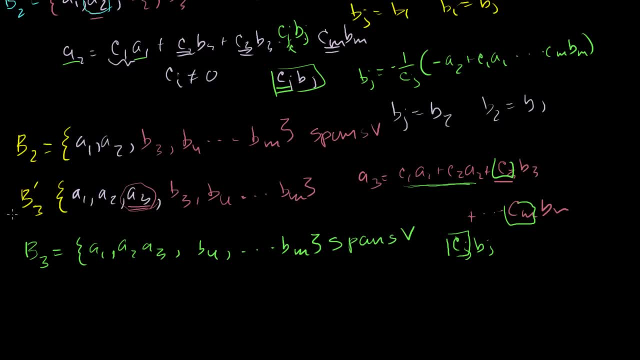 And I keep doing it. So what's going to happen eventually? What's going to happen If I keep doing this process over and, over and over again? eventually, I'll essentially replace all of the bm, Or I'll replace all of the n terms. 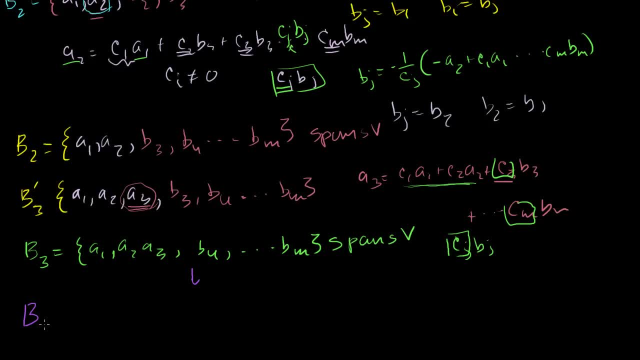 So eventually, I'll have a set that looks like this. I'll have a set that looks bm. Well, I will have replaced each of these guys with an a, Or I would have replaced each of these guys with an a. So I'll have a1, a2, a3, all the way to am. 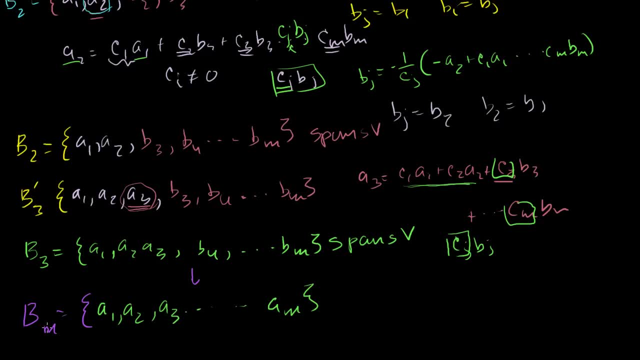 You can always do this by definition. if you started with that initial set b, that is a spanning set, And once you do this process, you'll get the same result: that this also spans b. Now let me write this: This is the result we got by starting off with a spanning. 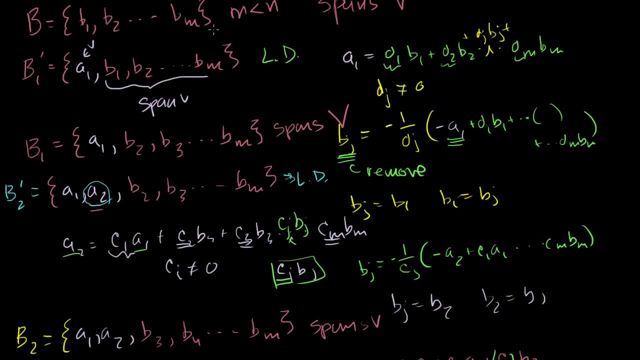 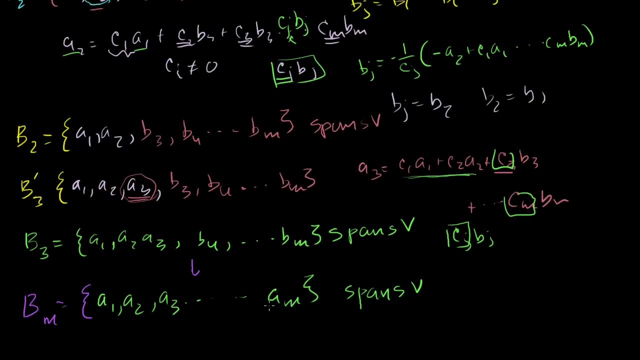 set b that has m elements where we said that m is less than n. So we always have enough a elements to do this, because we have more a elements than there were b elements to begin with, And we get the result that this spans v. 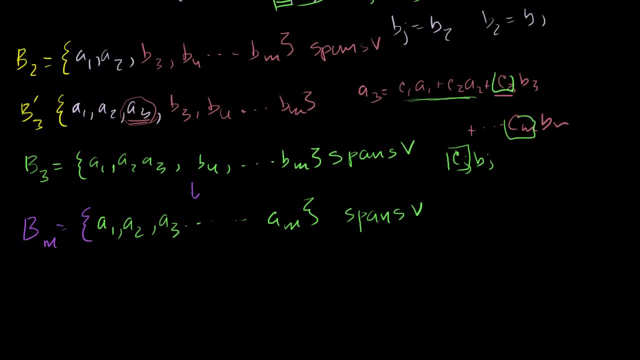 But we already said that the set a, which is equal to a1, a2, all the way to am, and then am plus 1. I don't know how many more terms there are between m and n, But then you go all the way to an. 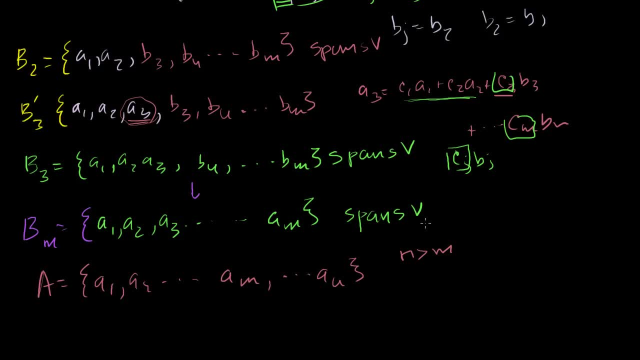 Remember we said that n is greater than m. Or when we defined b, we said that m is less than n. Same thing, that this was a smaller set. Now we're saying that this spans v, But at the same time we said that this was a basis. 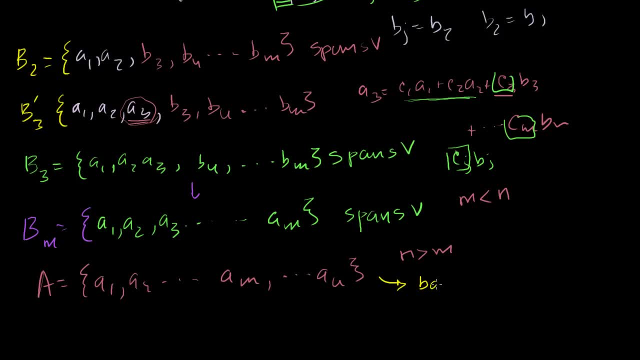 This was just our starting fact, that this is a basis for v Basis for v. Basis means two things: It means it spans v and it means it's linearly independent. Now, we just got this result by assuming that we had some. 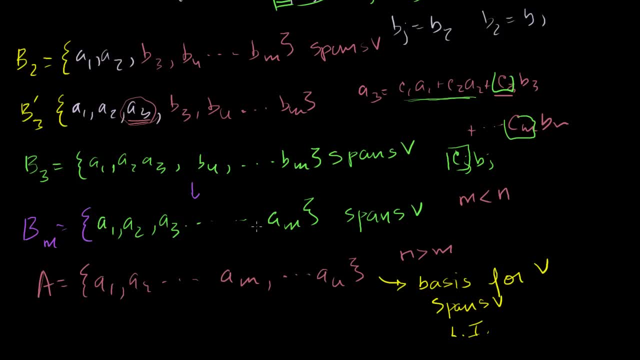 set b that's smaller than this set here that spans v. We were able to construct this by saying that a1 through am also spans v. So the result we got is that this spans v. But if this subset of a spans v, then 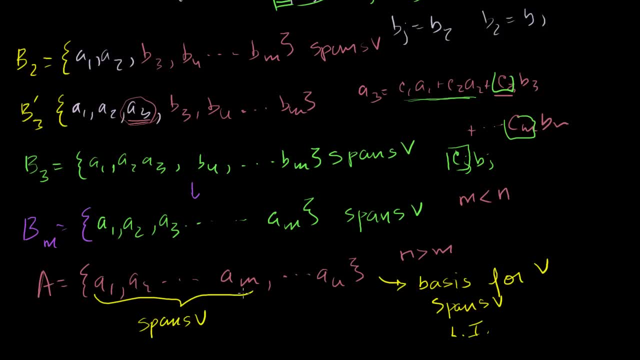 a1 spans v, Then a becomes linearly independent, Because if this subset spans v, that means that an can be represented as some linear combination of these guys. So that implies that you're linearly dependent, which is a contradiction with our original statement that set a is a basis. 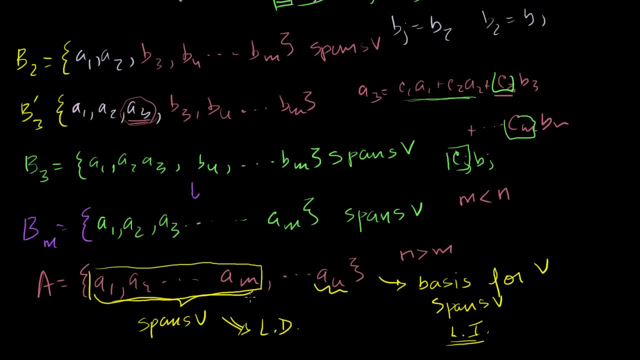 for v, because that means that it's linearly independent. If you're able to do this, then this means that this is: if there is some smaller spanning set, you get the result that a has to be linear. It has to be linearly dependent, even though we said. 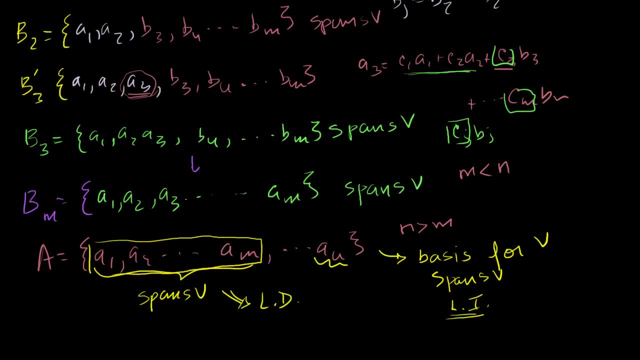 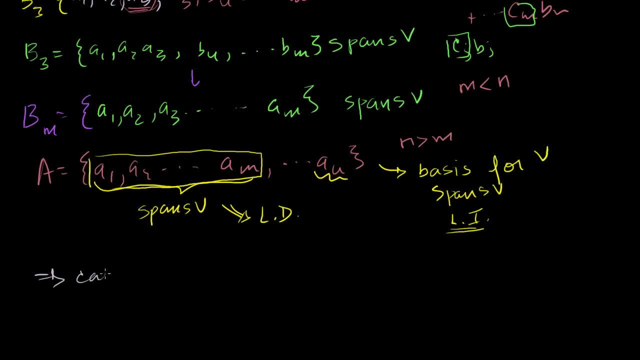 it was linearly independent. So we now know we get our contradiction. We say that there cannot be a spanning set b that has few elements than a. And this is a pretty neat outcome, because now if anyone tells you that, if I come up to you and I say, hey, I found. 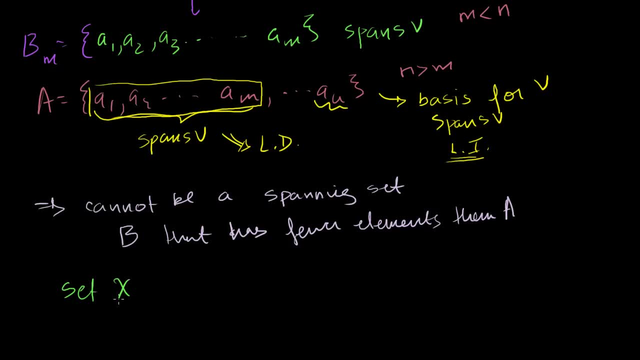 some set x. so set x spans the subspace. I don't know. let's just call that v again. then you know that an x has 5 elements. You now know that no set that spans the subspace v can have fewer than 5 elements. 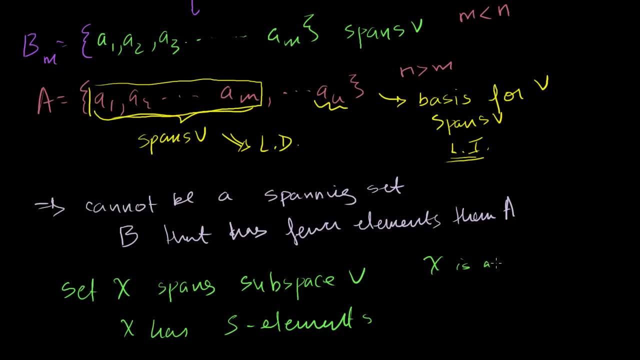 Even better if I told you that x is a basis for v and it has 5 elements, and y is a basis for v. y is another basis- my handwriting is degrading- y is- let me write it a little nicer. 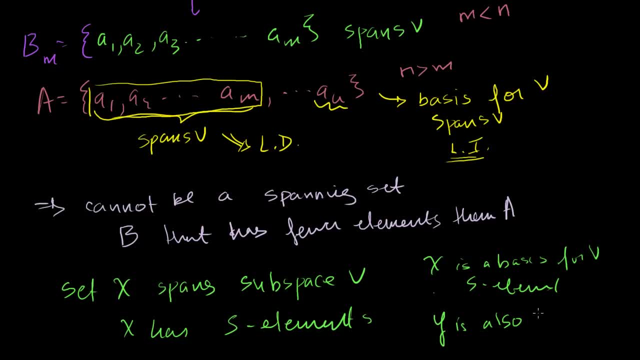 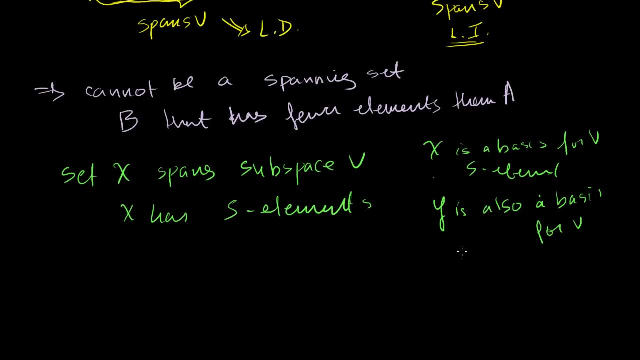 y is also a basis for v. So if I say that y is also a basis for v, you know that y also has to have exactly 5 elements. y has 5 elements. How do I know that? How do I know that? 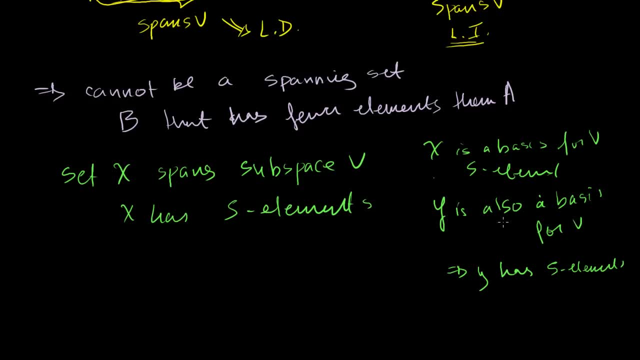 Well, if y is a basis, then it has to have. then that means that it spans v, And we know it can't have anything less than 5 elements. We just proved that. So one way we know that y has to have greater than or equal. 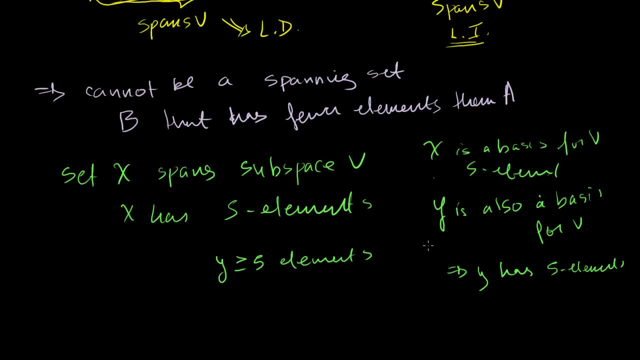 to 5 elements. But on the other hand, we know that if y is a basis for v and x is a basis, x also spans v. So we know that x has to have fewer elements than y. So we know that y has to have greater than x. or let me just 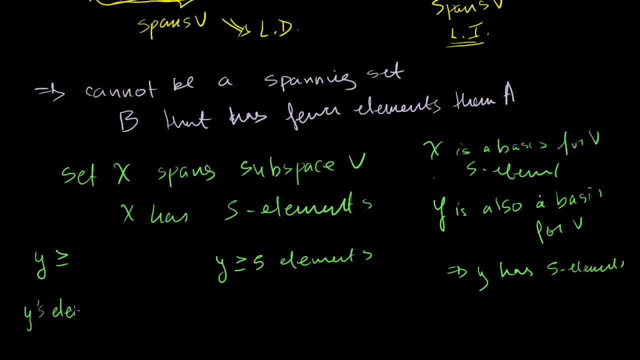 call it y's elements have to be greater than x's elements, Because any spanning set has to have more elements, Or at least as many elements as a basis set x's elements And then, since x is a spanning set, x's elements have to be. 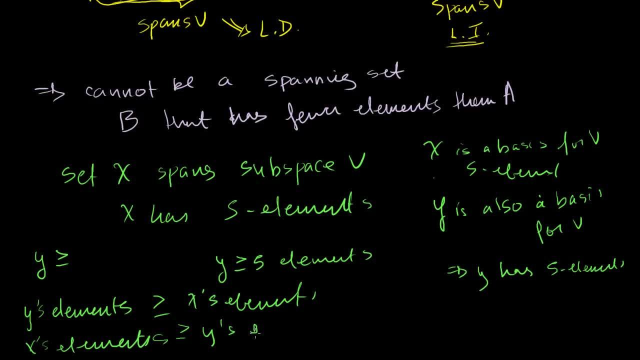 greater than or equal to y's elements, Because y is a basis- y's elements. I know you can't read that, But if this guy's elements are less than this guy's elements but it's also greater than or equal to- we know that x, the 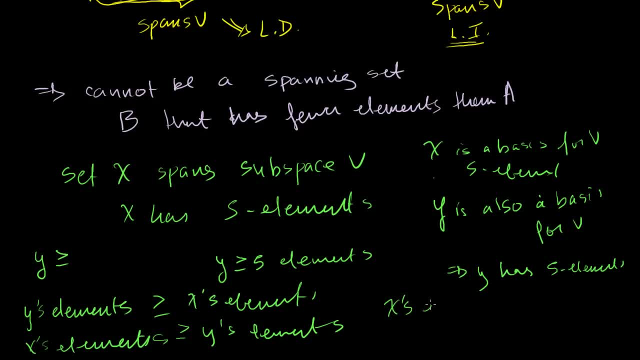 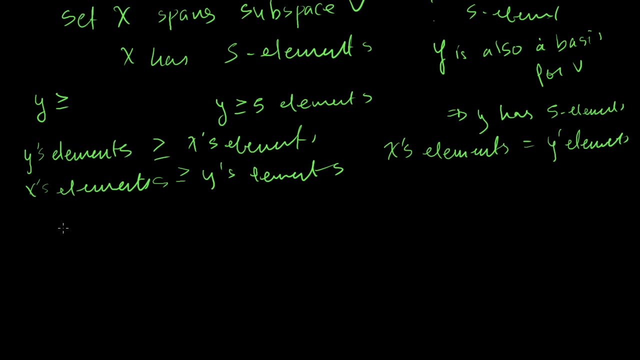 number of elements, that x has Elements, or the cardinality, or the number of elements in it, is equal to y's elements. And so, now that we know that, any basis for a vector space- so let's say that x, though let me just go back to our set a-